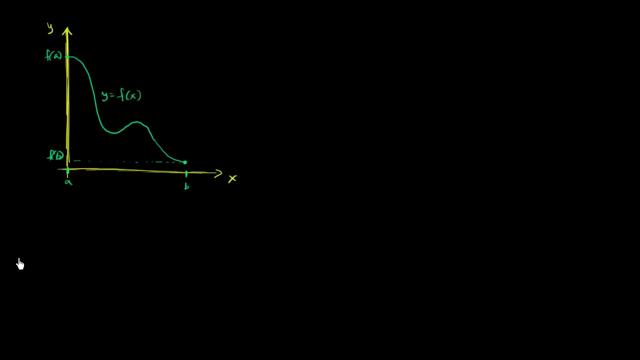 And it looks like a is equal to 0.. But you're probably thinking, hey, there are other kind of interesting points right over here. This point right over here it isn't the largest. We're not taking on this value right over here. 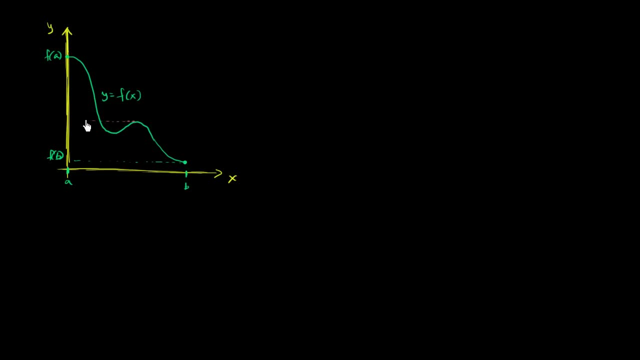 It is definitely not the largest value that the function takes on in that interval, But relative to the other values around it it seems like a little bit of a hill. It's larger than the other ones. Locally it looks like a little bit of a maximum. 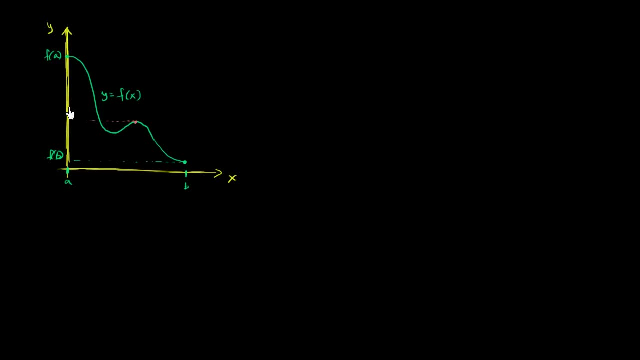 And so that's why this value right over here would be called. this value right over here, let's call this, let's say this right over here, is c, This is c, so this is f of c. We would call f of c is a relative maximum value. 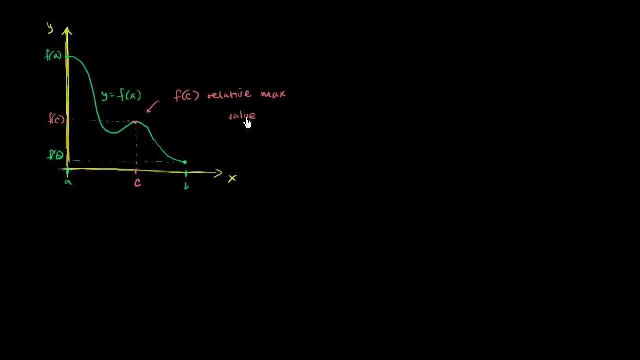 And we're saying relative because it's obviously- the function takes on other values that are larger than it. But for the x values near c, f of c is larger than all of those. Similarly- I can never say that word- Similarly, if this point right over here is d. 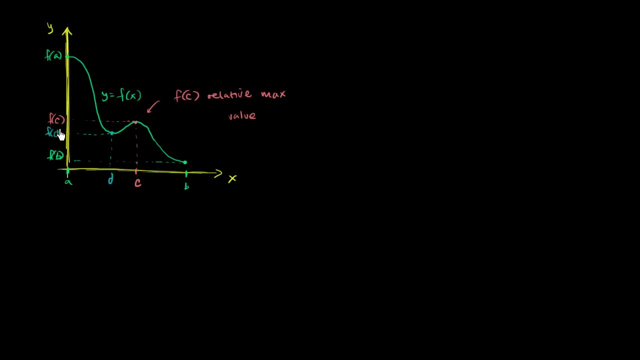 f of d looks like a relative. f of d is a relative minimum point or relative minimum value. f of d is a relative minimum or a local minimum value. Once again, over the whole interval there's definitely points that are lower. 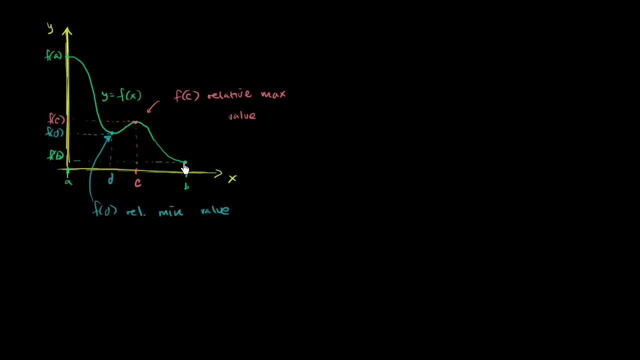 and we hit an absolute minimum, for the interval at x is equal to b, But this is a relative minimum or a local minimum because it's lower than the. if we look at the x values around d, the function at those values is higher. 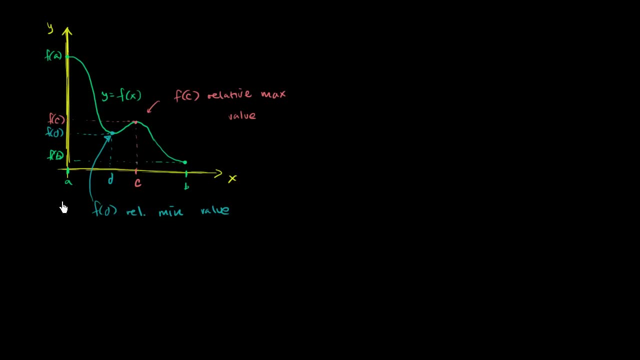 than when we get to d. So let's think about. it's fine for me to say: well, you're at a relative maximum, if you're at a larger, if you hit a larger value of your function than any of the surrounding values. 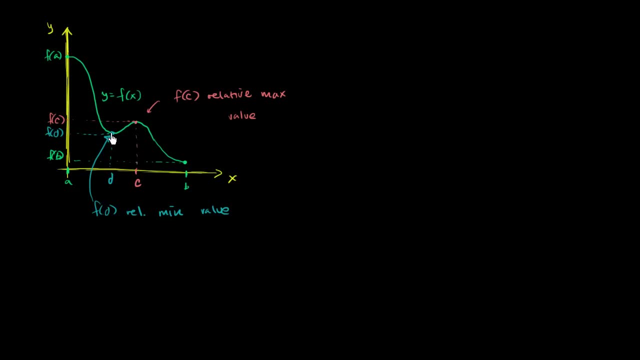 and you're at a minimum, if you're at a smaller value than any of the surrounding areas. But how could we write that mathematically? So here I'll just give you the definition. that really is just a more formal way of saying what we just said. 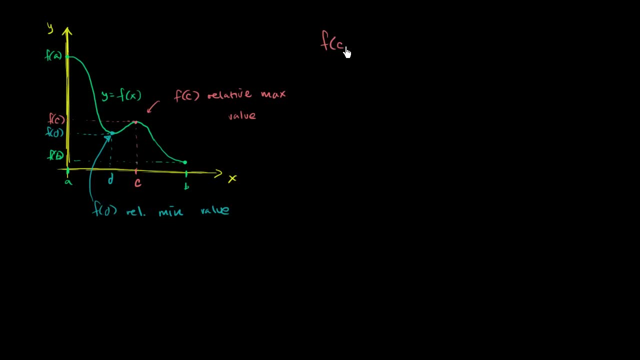 So we say, we say that f of c, f of c is a relative max, relative maximum value. if, if f of c is greater than or equal to f of x, for all x, for all x, that we could say, we could just say kind of in a casual way: 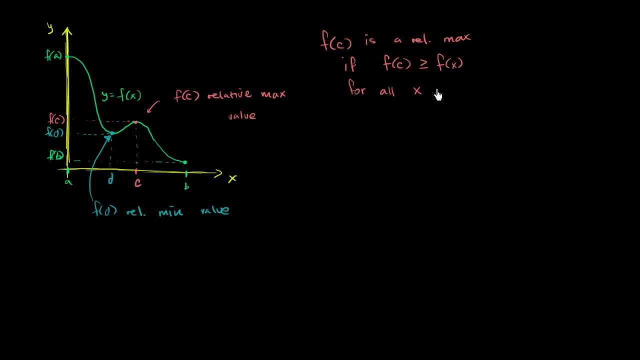 for all x near, for all x near c. so we could write it like that, but that's not too rigorous, because what does it mean to be near c? And so a more rigorous way of saying it: for all x, that's within an open interval. 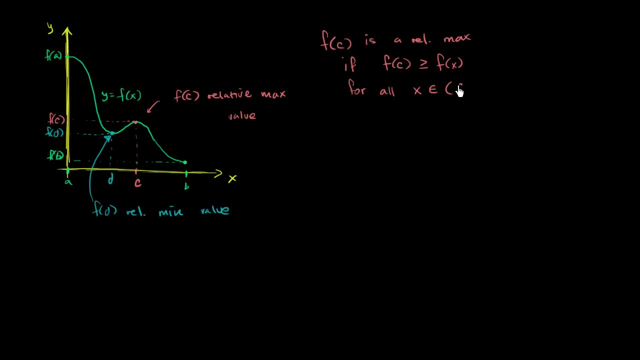 that's within an open interval of c minus h to c plus h, where h is some value greater than where h is some value greater than zero. So does that make sense? Well, let's look at it. So let's construct an open interval. 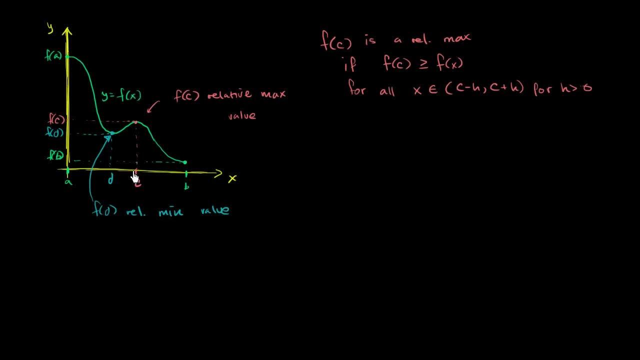 So it looks like for all of the x values in and you just have to find one open interval. There might be many open intervals where this is true, but if we construct, let's construct an open interval that looks something like that. So this value right over here is c plus h. 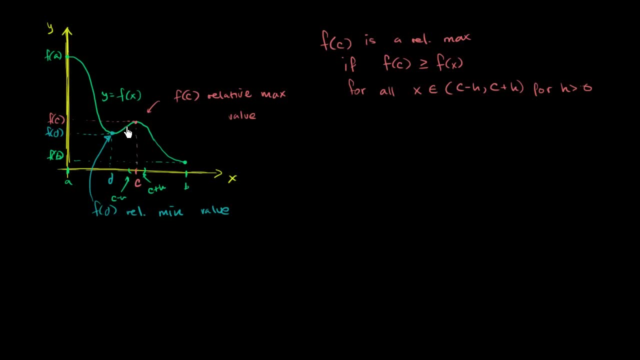 That value right over here is c minus h, And you see that over that interval the function at c, f of c is definitely greater than or equal to the value of the function over any other part of that open interval. And so you could imagine: 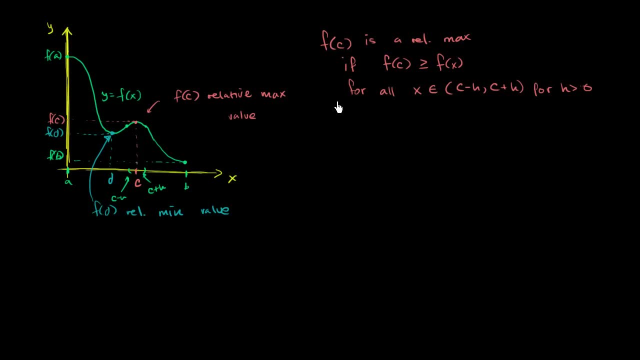 I encourage you to pause the video and you could write out what the more formal definition of a relative minimum point would be. Well, we would just write: let's take d as our relative minimum. We can say that f of d is a relative minimum point. 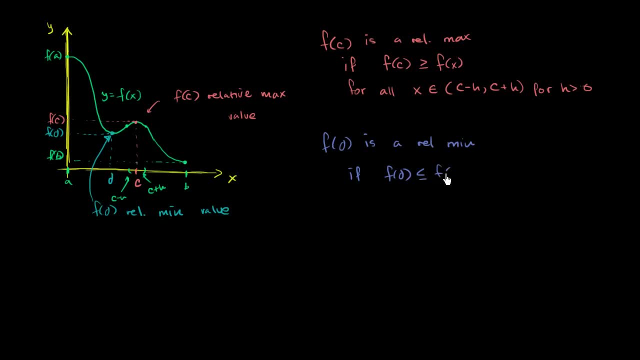 if f of d is less than or equal to f of x for all x in an interval, in an open interval between d minus h and d plus h, for h is greater than zero, So you can find an interval here. So let's say this is d plus h.